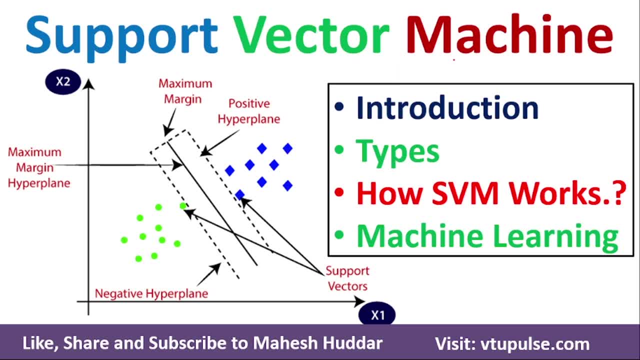 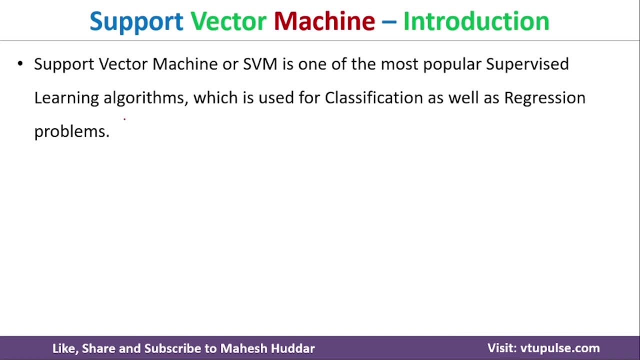 Welcome back. In this video I will discuss support vector machine in machine learning. Also, I will discuss what are the different type of SVM algorithms are there and how SVM algorithm works. Support vector machine, or SVM, is one of the most popular supervised machine learning. 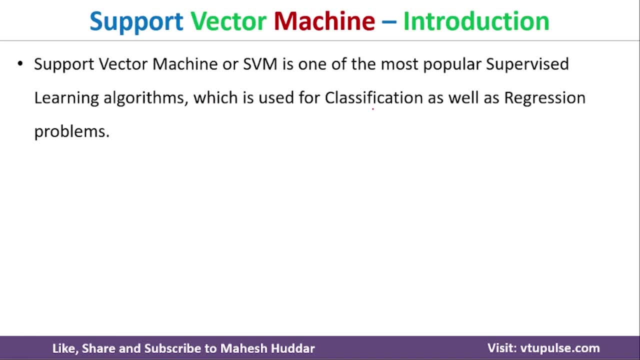 algorithm which are used to solve the classification as well as regression kind of problems. So in this case, first we need to understand what is supervised here. Supervised means in this case we need to give the label data as an input to this particular algorithm. 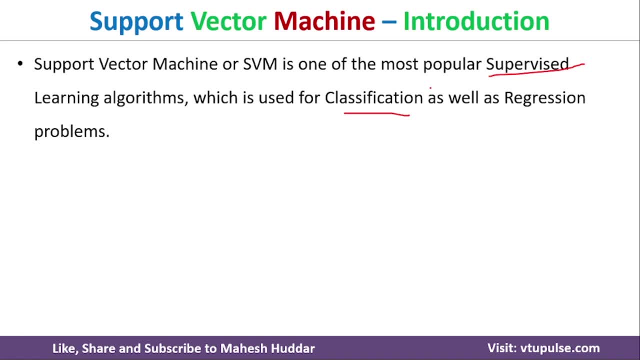 And what is classification? Classification problems are those where the target contains discrete number of possibilities. For example, if you want to solve a problem where we want to classify a mail as a spam mail or a not spam, in this case we have only two possibilities. 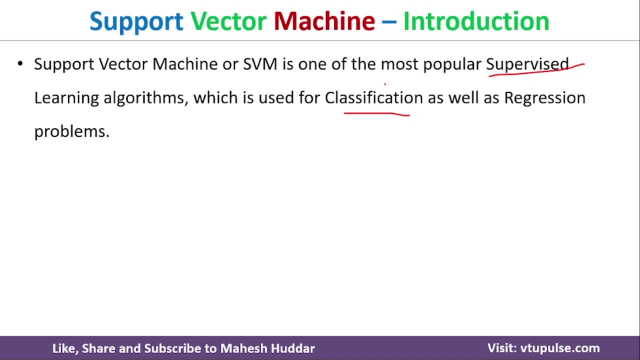 So such kind of problems are called as classification problems. But if the target label contains continuous values, such kind of problems are called as regression kind of problems. For example, let us say that we want to know the increase in salary of an employee based 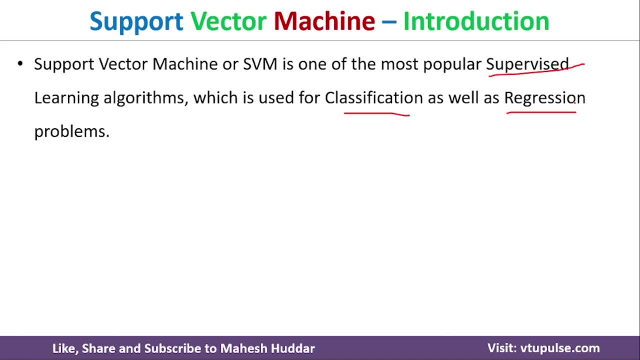 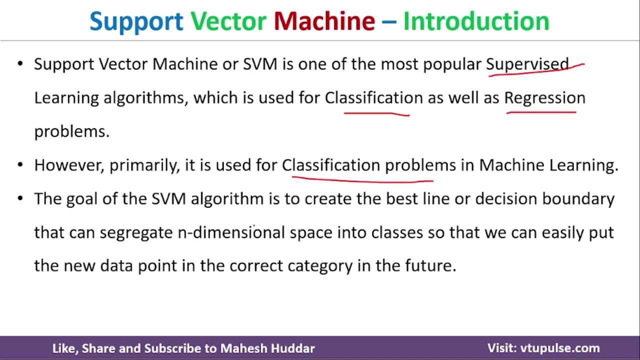 on his performance. In this case the increase in salary is a continuous in nature. Hence such kind of problems are called as regression kind of problems. Usually SVM or support vector machine algorithms are used to solve classification kind of problems in machine learning. The goal of 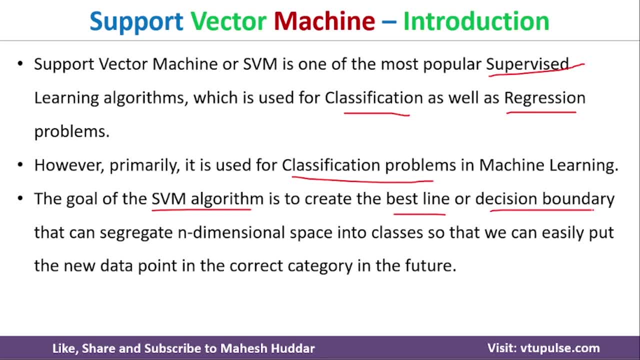 SVM algorithm is to draw a best line or a decision boundary to segregate the given data set into multiple number of classes. Once you draw that particular decision boundary. based on that particular decision boundary, we should be able to classify the new example into one of the classes. 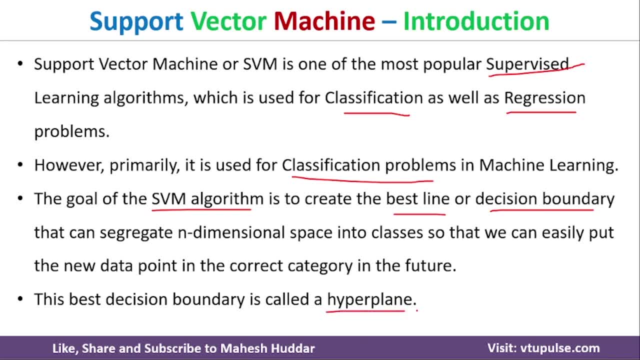 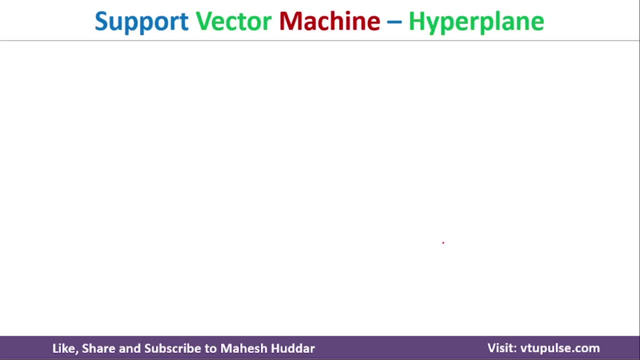 over here. Now this particular decision boundary is called as hyperplane in terms of SVM algorithm. Now the question comes in front of us is how to draw this particular hyperplane Given a data set. let us say that we have been given this particular data set, In this case. 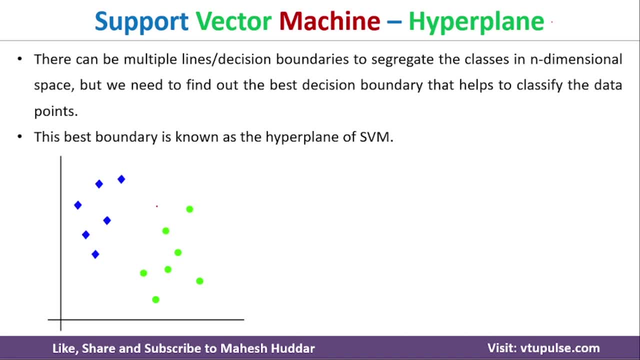 we have two classes. One is which is drawn in blue color and another one is drawn in- you can say that- green color. Now this particular data is linearly separable. We can draw a straight line and then we can separate this particular data into two classes. But which one is the best? 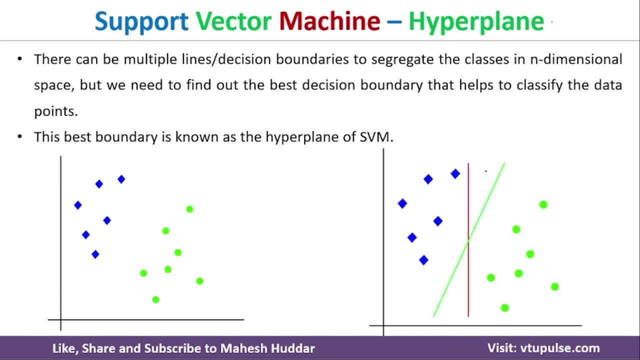 line over here, or the best decision boundary, Because if you look at this particular diagram, I have drawn two lines, one with red color, another one with green color over here. Between these two, which one I supposed to select? So what we need to do over here is we need to draw all possible lines, The one which is having 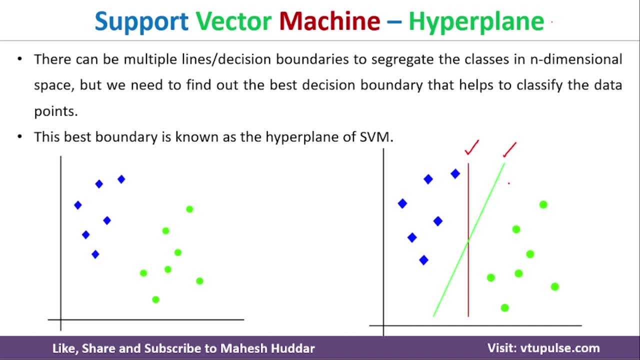 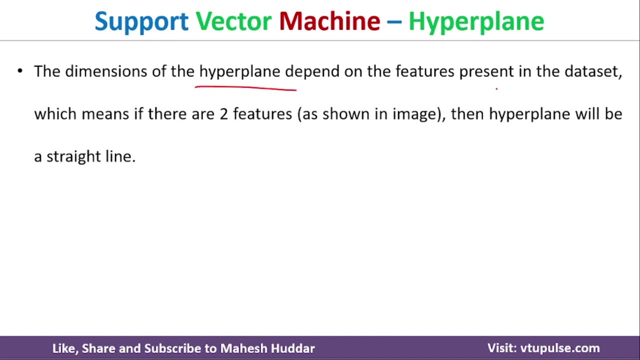 the best accuracy that particular line we need to select. that will be called as the hyperplane over here. The dimension of this particular hyperplane depends on the features present in that particular data set. For example, we have only two features. Let us say that we have x and y. 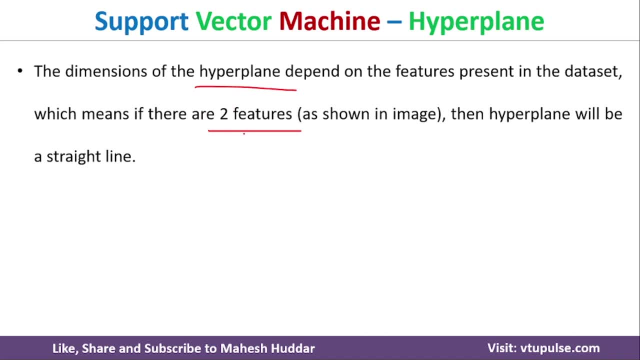 In such case we will be able to draw a straight line and then we can classify that particular data. So in such case the hyperplane will be a straight line. But if you have more than two data features- for example we have three features or more than three- 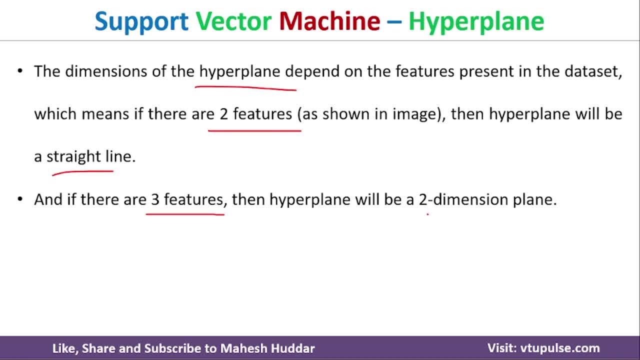 features. in such cases, we cannot draw a straight line. We need to draw something called as a plane or something like that That will be called as the hyperplane in this case, or a two-dimensional hyperplane over here. But very important thing is, we need to draw a hyperplane in such a way that 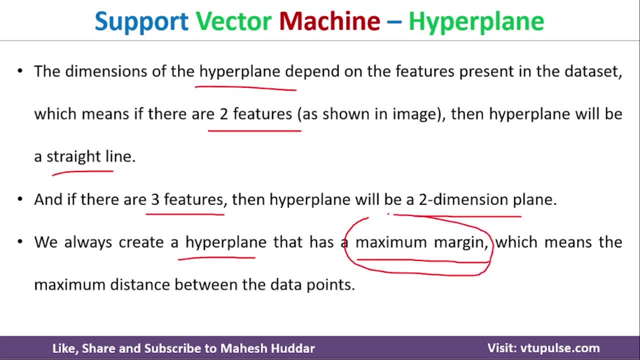 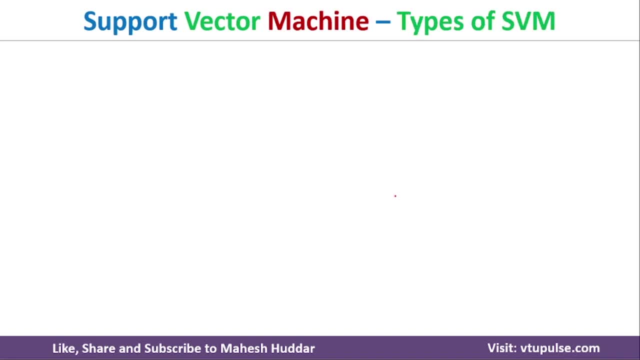 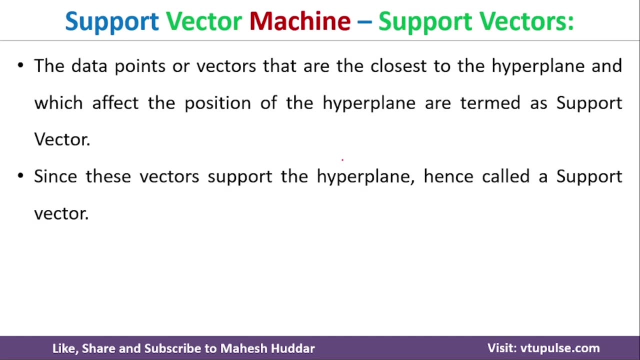 we will get the maximum margin. I will discuss this particular maximum margin in detail at the later stage. For this particular hyperplane, we use to consider two things over here. This one is the nearest point on both the sides. For example, if you go with this particular data set, this particular 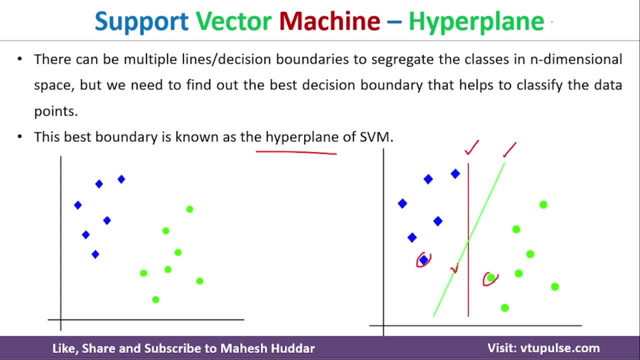 point and this particular point are nearest for this particular hyperplane. So these two are called as the support vectors in this particular case, For this one, this one is the nearest one and this is the second nearest one. This one and this one will be called as a support vector for. 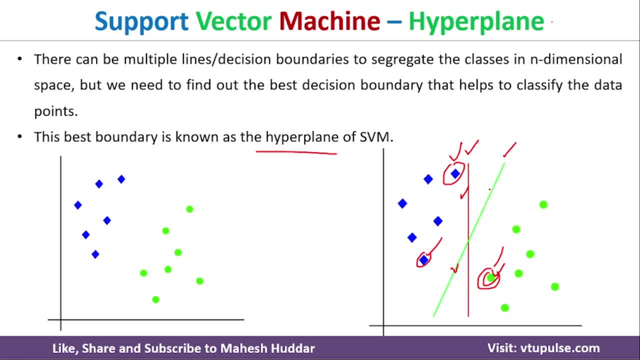 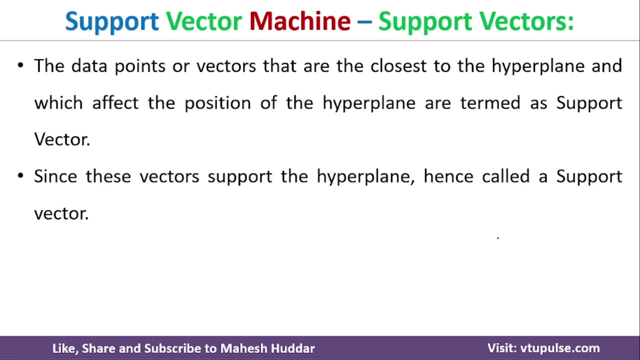 hyperplane, but based on the maximum margin, we will select between these two things, but, end of the day, the one which is having nearest data point for that particular hyperplane, that will be called as the support vector over here. now coming back to the next part of our discussion, that is what? 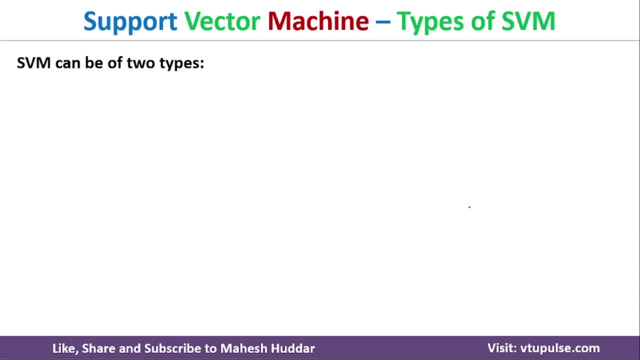 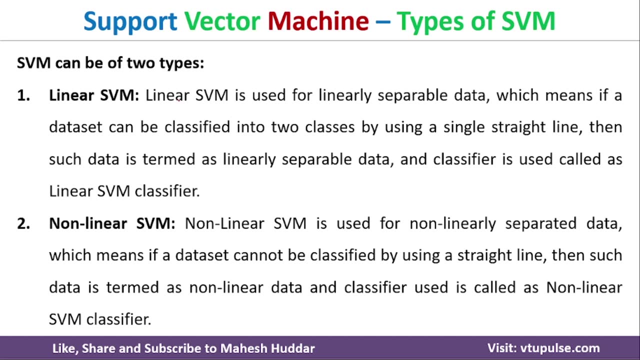 are the different type of svm are there? there are mainly two type of svm we have. one is called as linear svm, another one is called as non-linear svm. the linear svm is one where we can separate the data with the help of a straight line. for example, we have been given a data and we can 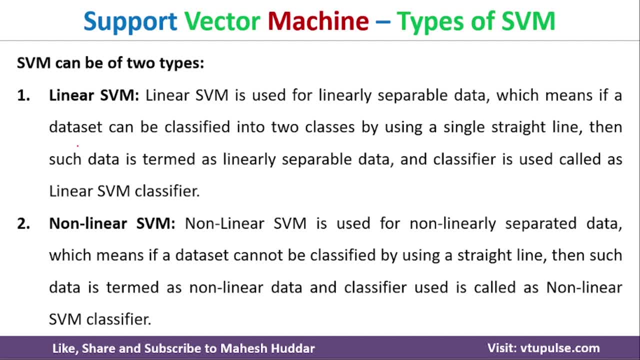 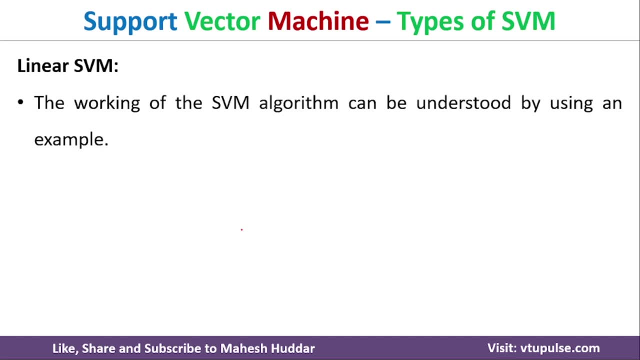 separate that particular data with the help of a straight line. such kind of svm is called as linear svm. if we are unable to draw a straight line to divide that particular data set into classes, such kind of svm is called as non-linear svm, for example. i will consider one example to understand this linear svm in detail. let us say that this is a 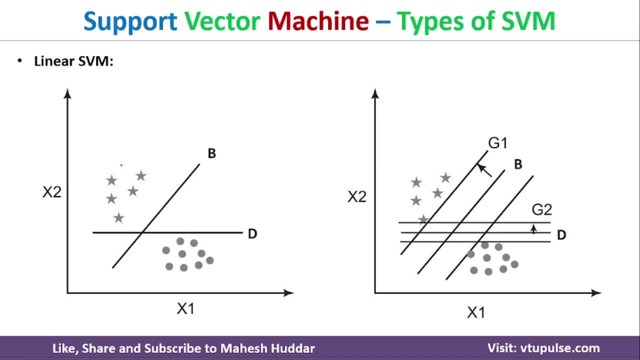 data set given to us. in this case, one class of data is drawn with star color. another set of data is called as is drawn with the circle over here. now this particular data can be separated with the help of straight line. hence it is called as the linear svm over here. but the question comes. 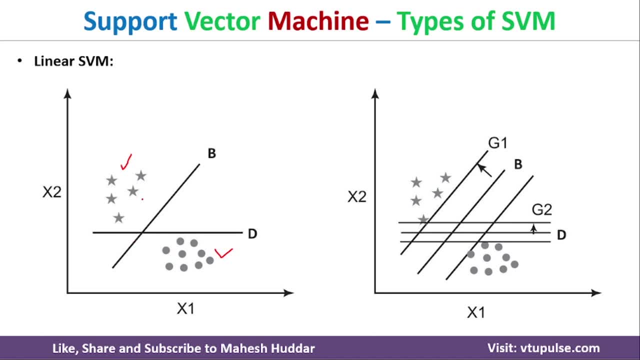 in front of us when we draw multiple number of straight lines to separate this particular data. which particular straight line should be considered as a hyperplane over here so that can be understand with the help of this particular diagram? what we do over here is, for example, if you 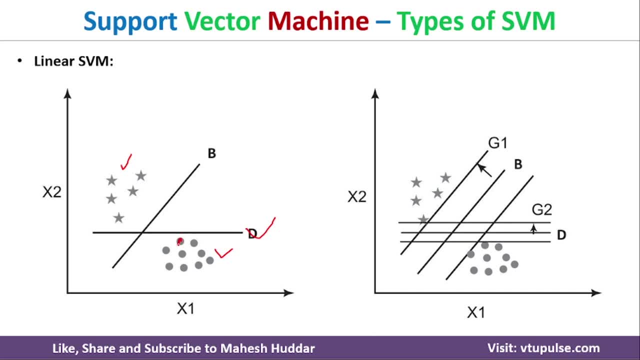 consider d as a hyperplane for this one, this one and this one will become the support vectors over here. so we need to draw a parallel line which will test this particular support vectors and they are parallel to what we can say, that our hyperplane and then this distance we need to. 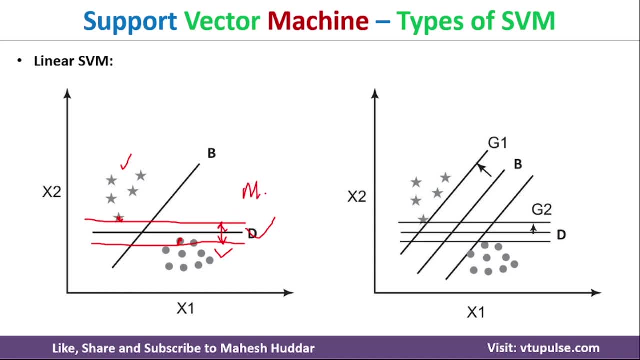 calculate so this distance. you can say that it is a hyperplane, and this distance we need to calculate is m1. similarly, we have to do it for this particular b. also, for this particular b, this will become one support vector and this will become another support vector we need to draw. 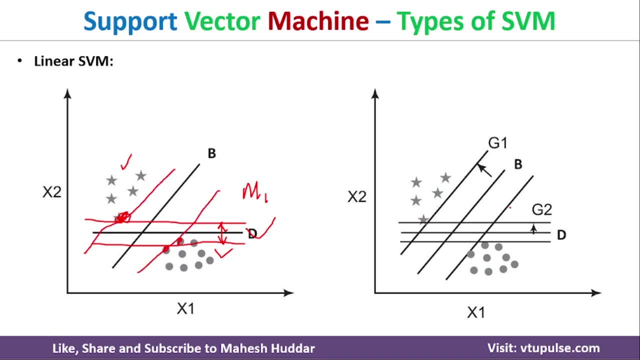 a straight line over here. we need to draw a straight line over here. i have drawn it here correctly. and then we need to calculate this particular margin over here. now let us say that this margin is equivalent to m2. now if we compare this m1 and m2, the margin m1 is smaller compared. 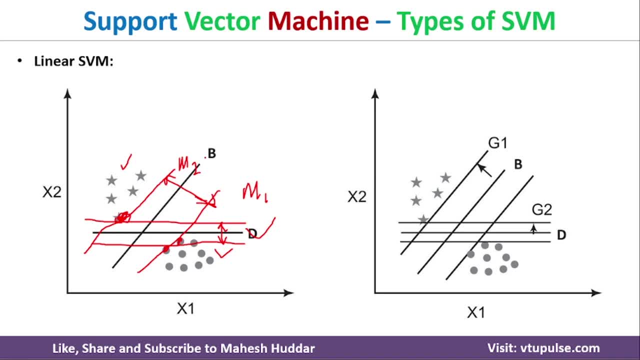 to this m2. so we can say that between these two, this particular b is the best line which will divide this particular data set into two classes over here. so b will be considered as the hyperplane in this particular case over here. but it may not be the case all the time, because we need to do it for all possible. 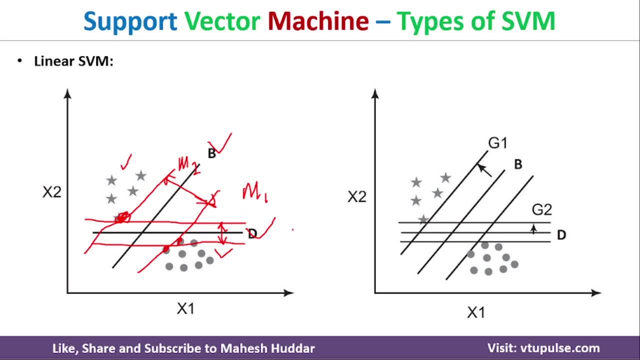 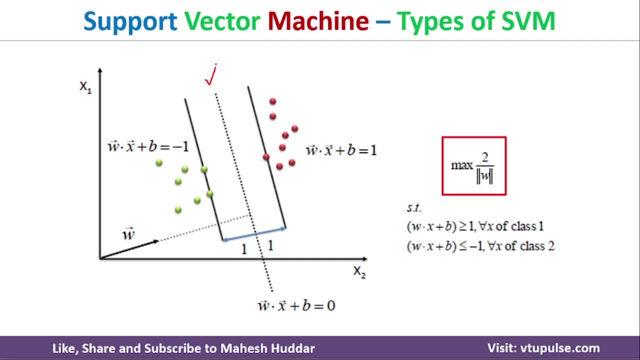 lines, the one which will give you the maximum margin that should be considered over here. the calculation of this particular maximum margin can be shown mathematically something like this: let us assume that this is your hyperplane and this is the first support vector and this is a second support vector. what actually happens over here is for 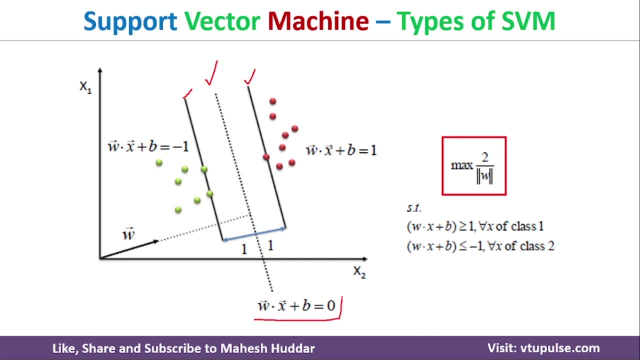 this particular hyperplane, we will write this particular equation, that is: w into x plus b is equal to zero. now, when i write something like this on this particular side, on one side for this particular support vector, we will get w into x plus b is equal to minus one. on another side, we 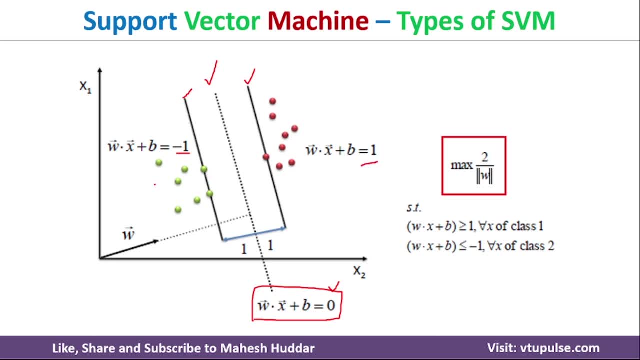 will get plus one. if you go beyond this particular thing, it will be less than minus one. if you go beyond this side, it will be greater than or equivalent to one over here. because of that, from here to here, we will get distance one. from here to here, we will get distance one for each and every. 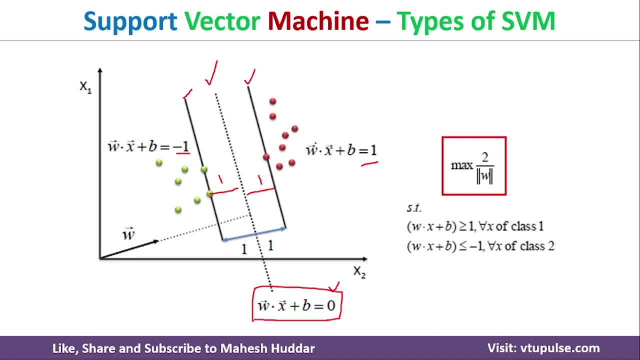 what we can say that the support vectors. so what we need to do over here is we need to get an hyperplane where we will get the maximum value for this particular condition, that is, two divided by cardinality of w. if we get this particular maximum value for that particular w should be considered. 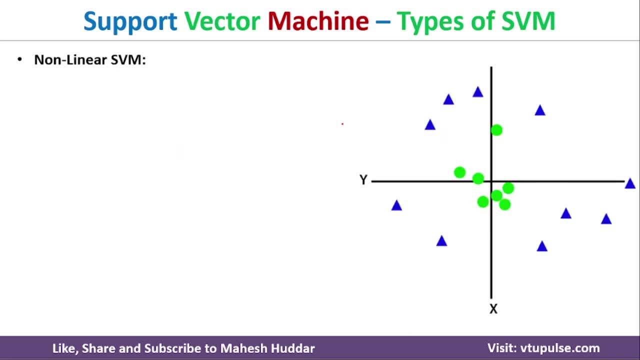 we can say that the final hyperplane over here, the next type of svm is called as non-linear svm. this non-linear svm is one where we will not be able to draw a straight line to divide this particular data into two classes over here. if you look at this particular thing, if i draw anywhere, 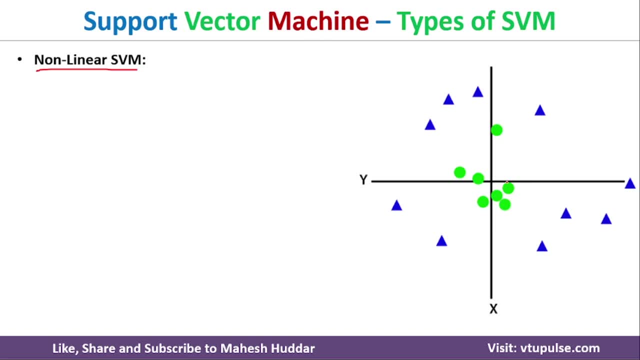 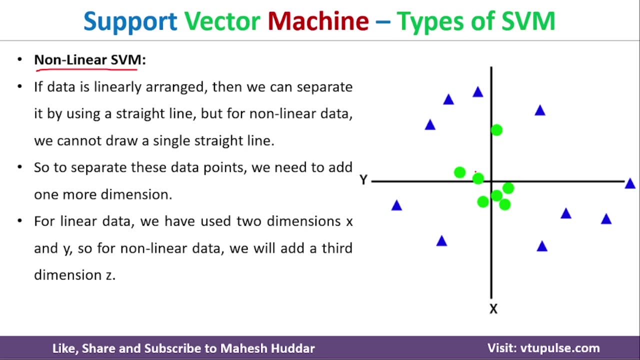 a straight line. i will not be able to classify this particular data into two classes here, so what i need to do is i need to convert this particular data into what is that called as linear data. for that reason, we can use some thing called as a mapping functions or something like that. in this case, i have used one mapping.